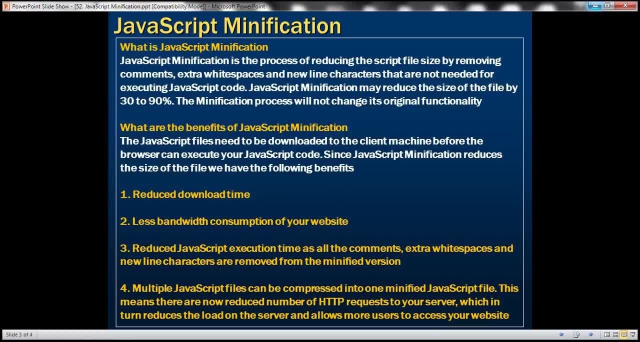 JavaScript minification may reduce the size of the file by 30 to 90 percent. The minification process will not change its original functionality in any way. What are the benefits of JavaScript minification? The JavaScript file needs to be downloaded to the client machine before the 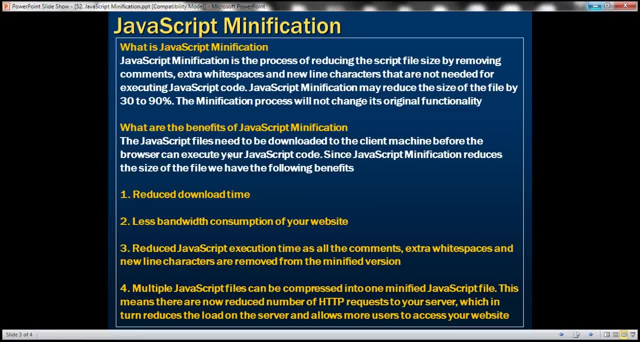 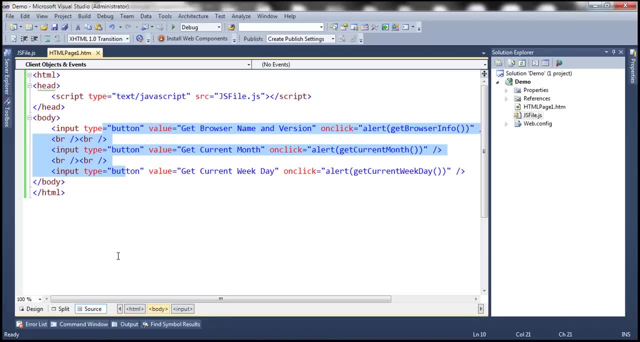 browser can execute your JavaScript code. Let's understand what we mean by this statement. Here we have an HTML page with three buttons. When we view this HTML page in a browser, this is how it looks like. When we click this button, get browser name and version it displays. 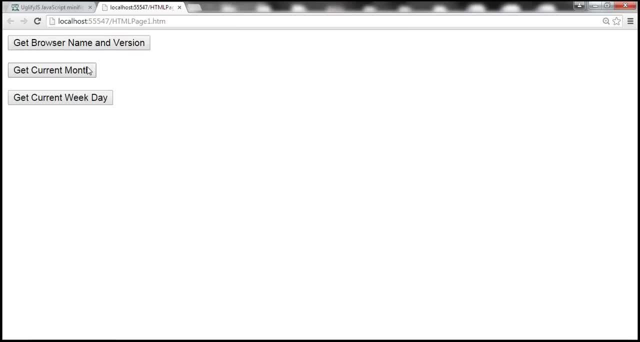 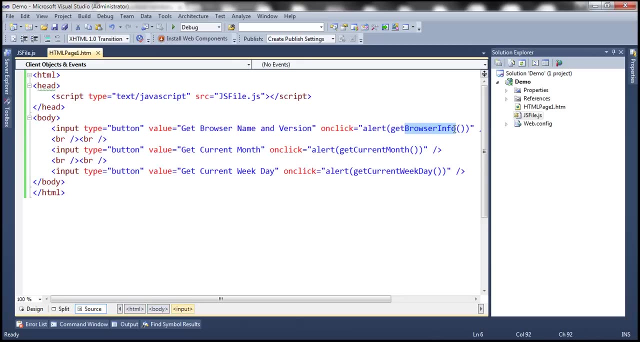 the browser name and version. When we click get correct month, it displays the current month. get current weekday: displays the current weekday. all this is achieved using JavaScript. now notice: when we click this button get browser name and version, we're calling get browser info JavaScript function. when we click get current month, we're calling get current. 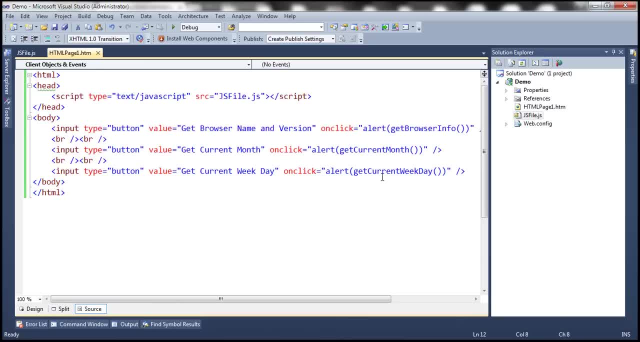 month function. get current weekday. we're calling get current weekday function. where are all these functions present? notice: within the head section we have a script reference. we are referencing an external JavaScript file with name jsfilejs. this is present in our project folder and this JavaScript file. 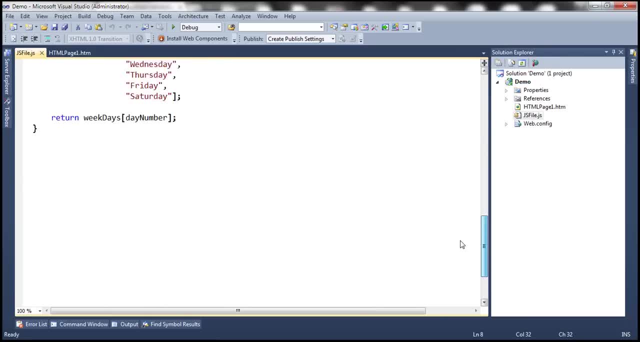 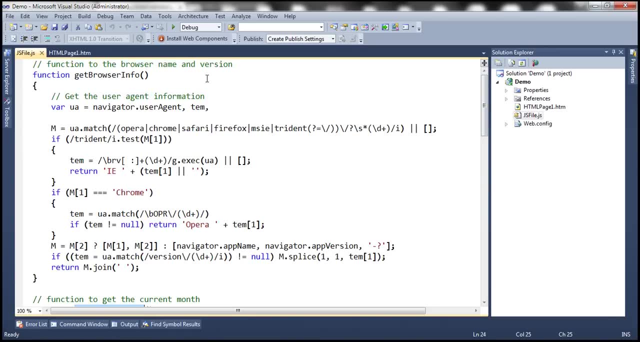 has got all those three JavaScript functions. notice we have get current weekday, get current month and get browser info. now, when a client makes a request to this page, HTML page 1, dot. HTML, along with the name of the file we're calling: get current weekday. we're calling: get current month and get browser info. now, when a client makes a request to this page, HTML page 1, dot. HTML, along. 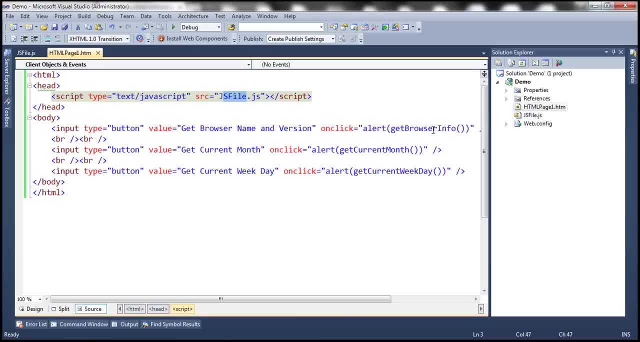 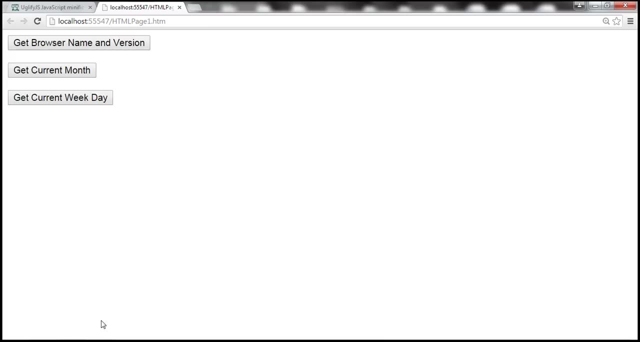 with the pages HTML. it also needs to send this JavaScript file, jsfilejs. so this JavaScript file need to be downloaded to the client machine so the client browser can execute the JavaScript functions right. so that's what this statement means: the JavaScript file needs to be downloaded to the 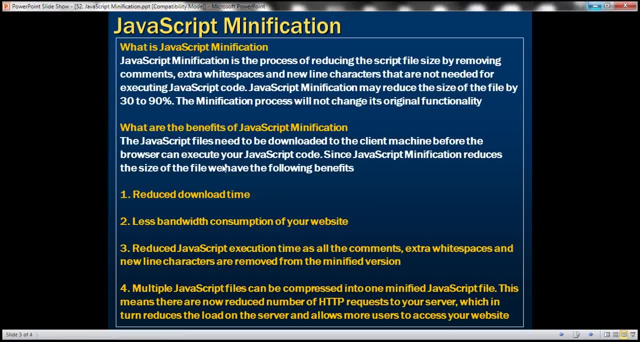 client machine before the browser can execute your JavaScript code. since JavaScript minification reduces the size of the file, we have these benefits: reduced download time, less bandwidth consumption of your website. reduced JavaScript time as well, because all the comments, extra white spaces and new line characters are removed. multiple JavaScript files can be. 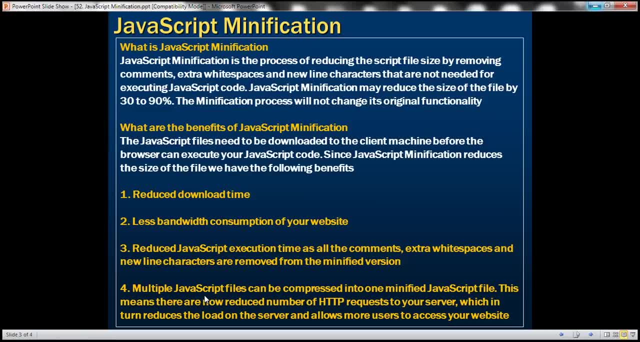 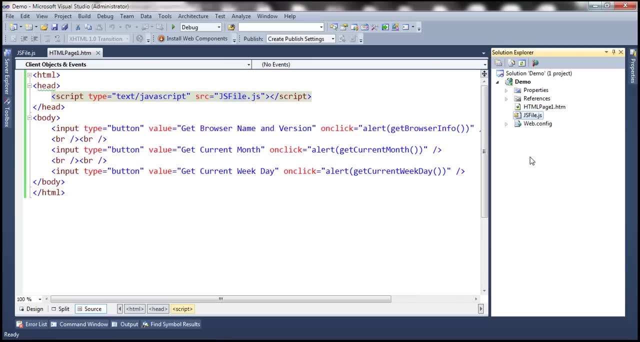 compressed into one minified JavaScript file. this means there are now reduced number of HTTP requests to your server, which in turn reduces the load on the server and allows more users to access your website. let's say, within our app application, we've got four different JavaScript files. this means this client: 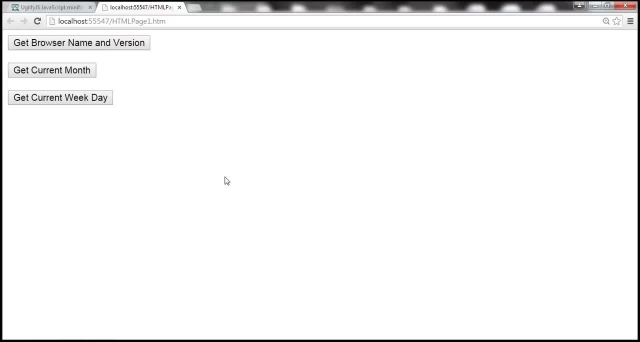 browser have to make four different HTTP requests to download all those four files. now if we combine all those four JavaScript files into one JavaScript file and if we minify that, then the client browser needs to make just one HTTP request, which means there is less load on the server. that means the server. 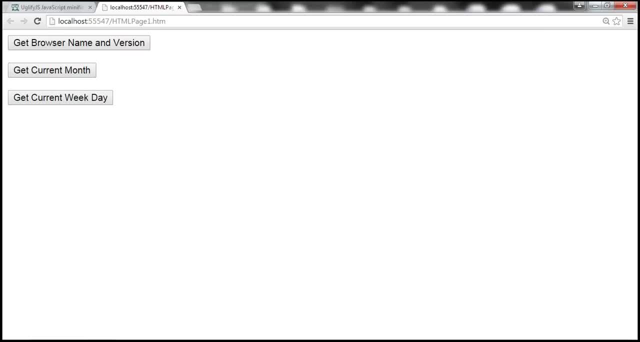 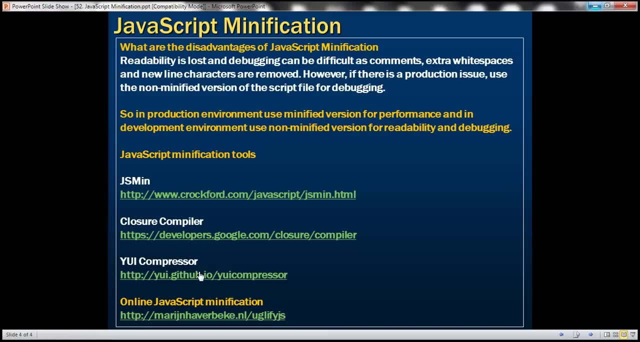 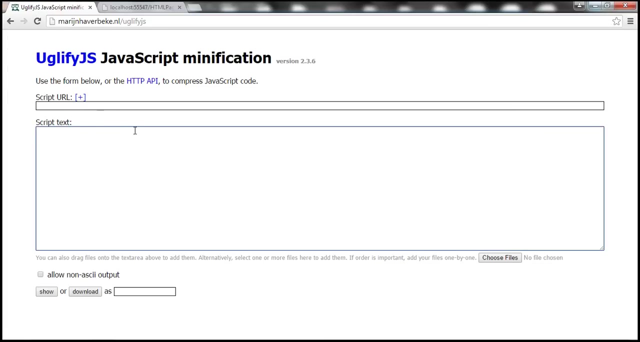 can now process more requests. now let's look at the process of JavaScript minification. there are several tools available, as you can see here now. there are also several websites that provide online javascript modification, and here is one such website. now, when we visit that website, so we can paste our JavaScript text here and then minify it. 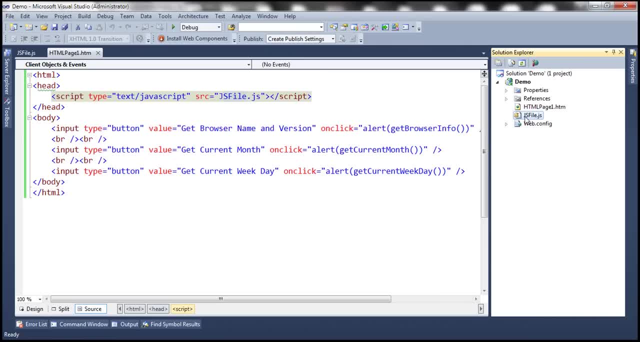 so let's go to our JavaScript file. so, before we minify that, let's open the project for java files. and open up the project for java files. it comes with the java files, so let's go to that. java files with the java files, let's open the project. 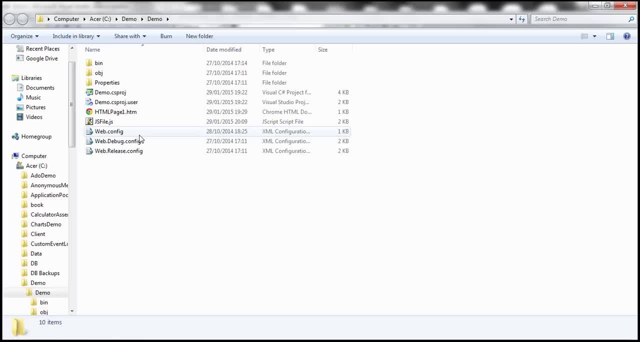 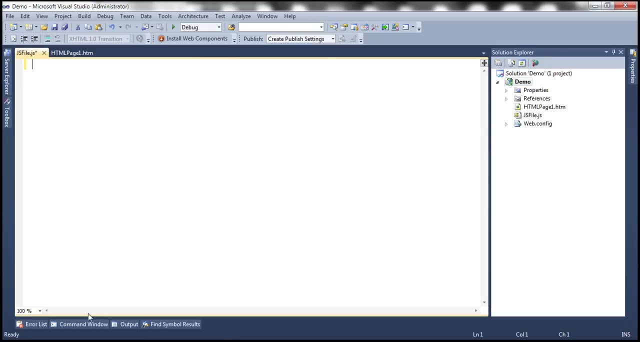 folder in Windows Explorer. and if you look at the size of this file, notice that the size is 1.66 kilobytes. right, so now let's go ahead and cut this entire JavaScript file from this file and paste it within this text box. so now, if you 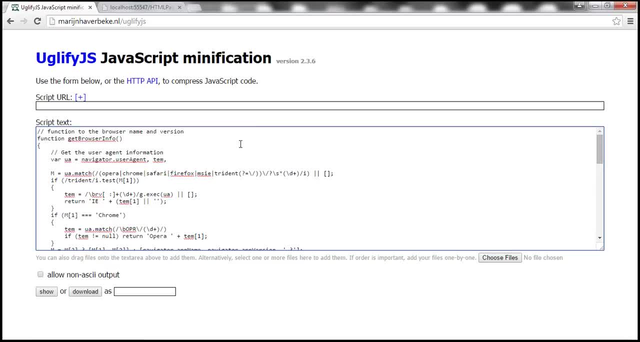 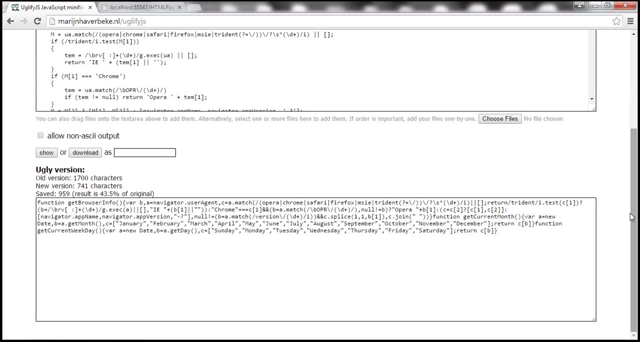 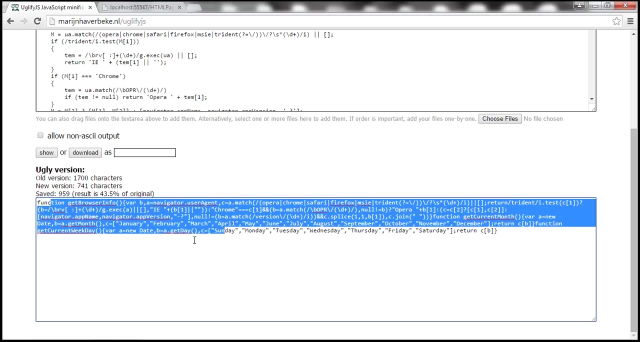 look at this JavaScript code. it's very readable because you've got comments. you've got, you know, white spaces, new line characters, so it's easier on the eyes. it's easy to read. now let's go ahead and minify it. notice that this is how the minified version looks like. now, this is not easy to read. it's not easier. 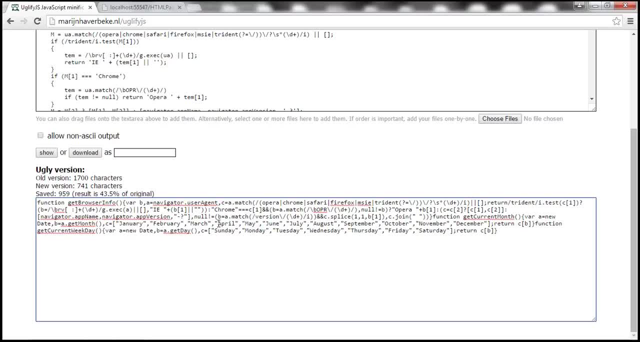 on the eyes, it's not easy to debug as well. okay, we'll look at that in just a bit. now look at the statistics here. the old version of our script had a 1700 characters. the new version has only 741 characters, and if you look at this,